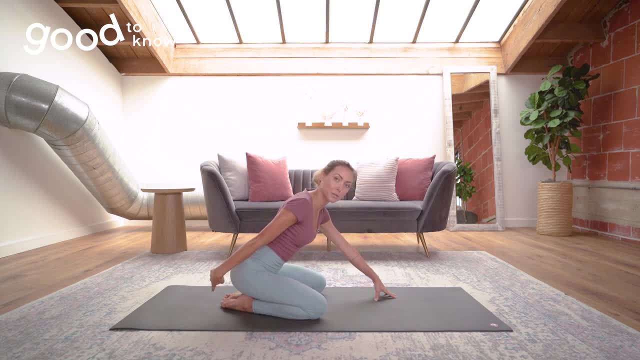 bring your big toes to touch and allow your seat to drop towards your heels. It may or may not connect, Don't worry about it. Now, the further that your knees are spread, the deeper this becomes an opener for your hips. So take it slowly as you begin to walk your arms forward. 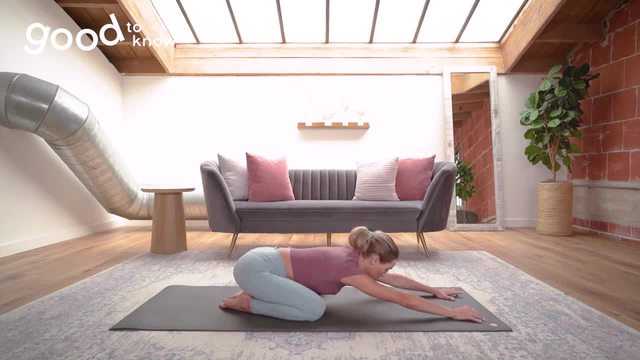 and then you decide if you want to turn up or turn down the volume. So allow your forehead to melt down towards the mat Again. it may or may not connect, and that's okay. But now immediately bring your awareness to your hips. 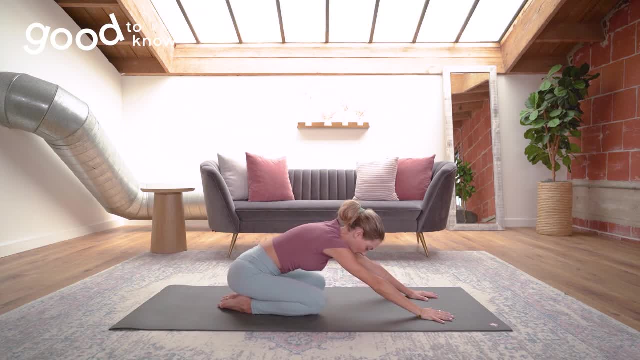 and notice. if it feels like too much, you can press on your palms, bring your knees a bit closer together, Or if you want a little more, you can take your knees a little wider. Now, if this is too much sensation altogether, then a nice alternative is to bring your 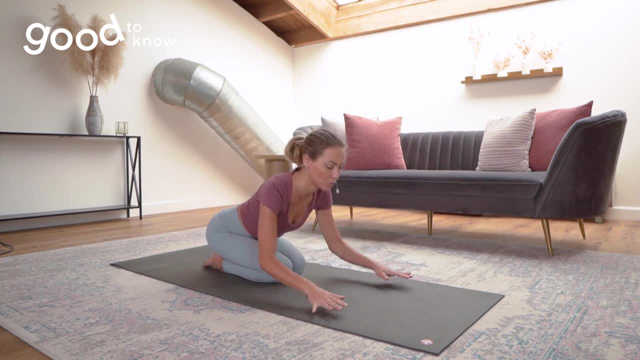 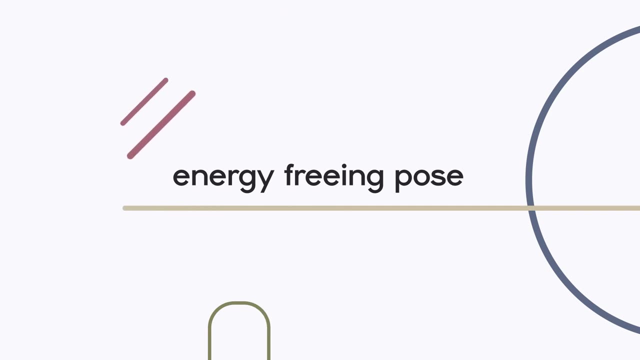 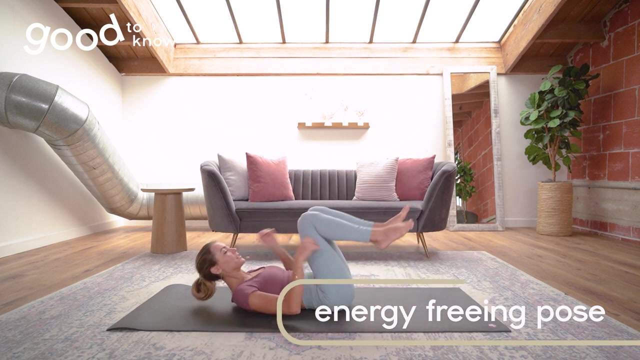 inner thighs and knees to touch and then drape your torso down over your hips. There you have it: child's pose. The next pose is energy-freeing pose, or knees into chest. So you'll make your way onto your back and hug your knees into your chest. Now you'll notice right. 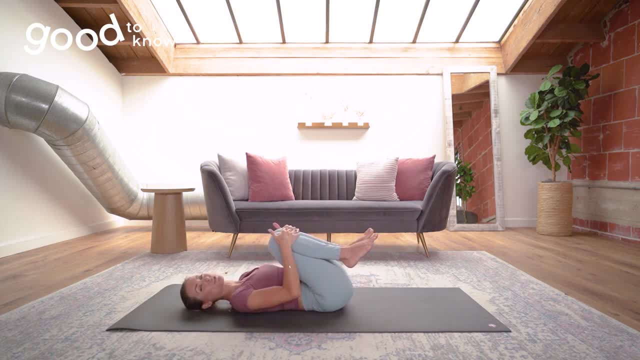 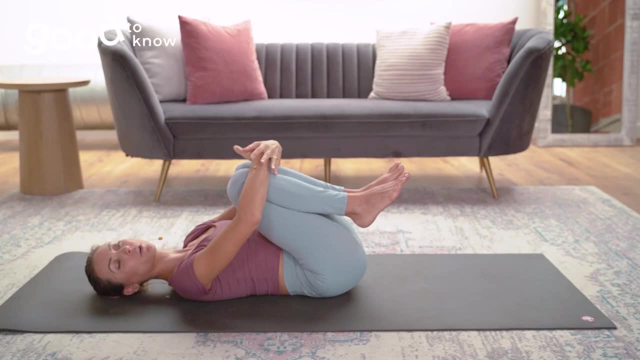 away how tight your hips feel, based on how close you're able to draw your thighs towards your stomach. Don't worry about it, Just get a good grip of your knees, whether that's with your hands. maybe you can grasp opposite wrists or forearms working to one day. maybe. 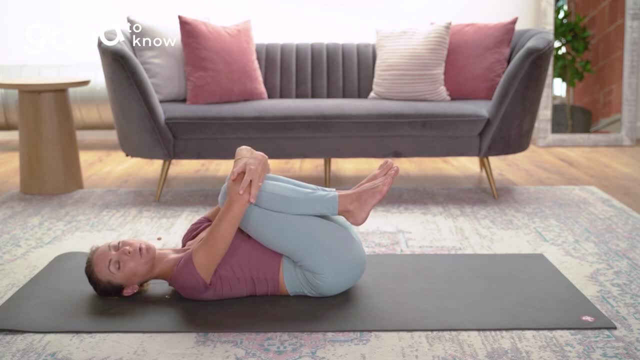 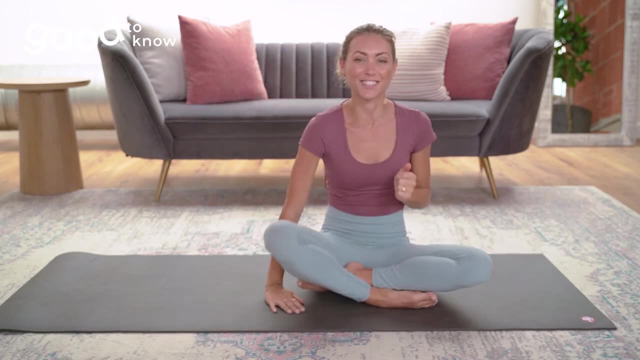 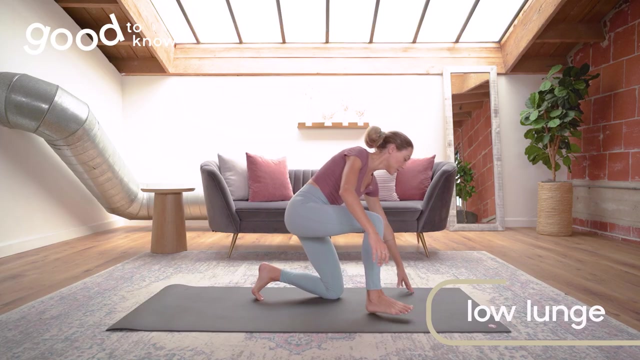 clasp opposite elbows, but just breathe deeply. wherever you are today, Usually you want to stay in this pose for several breaths. So there you have it. That was knees to chest. Our next pose is a low lunge. So you'll experience this pose in a lot of yoga classes. To do it, you'll bring. 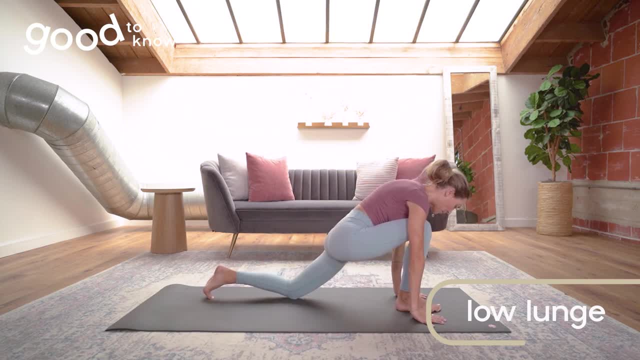 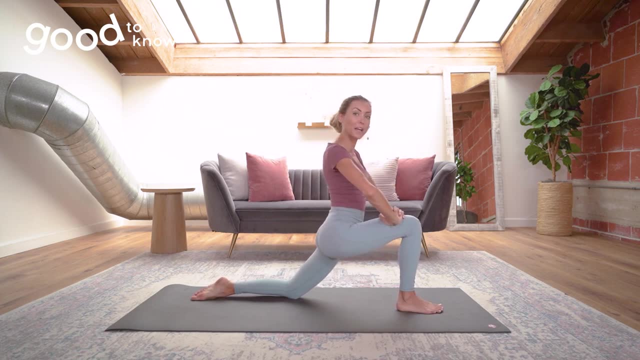 your foot between your palms, extend your back leg long and then come up when you're ready. And for this pose today we're going to try interlacing fingers on top of thigh, And what I like for this pose is to try interlacing fingers on top of thigh, And what I like 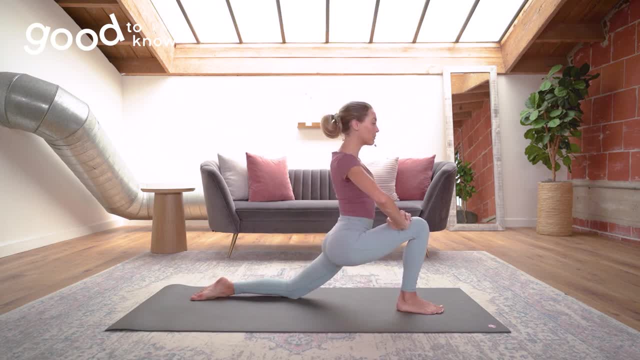 for this pose is to try interlacing fingers on top of thigh, And what I like for this pose is to For this hand placement for your hips is it allows you to melt your hips forward and down and just breathe here. Try to stay for five to 10 breaths and then do the opposite side. 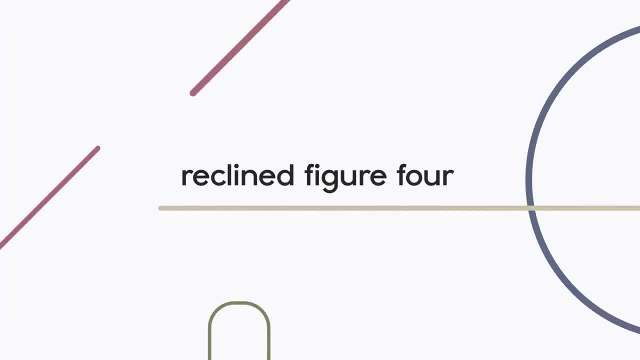 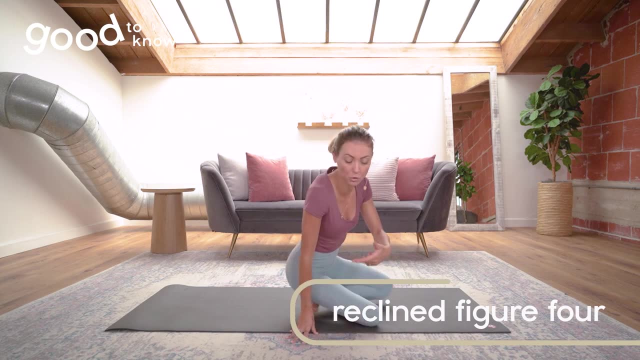 So there you have it, low lunge. Our next pose is a reclined figure four pose. What I love about this is it tends to be a more accessible version of pigeon pose, which you'll commonly see taught in yoga classes. So for a reclined figure four.